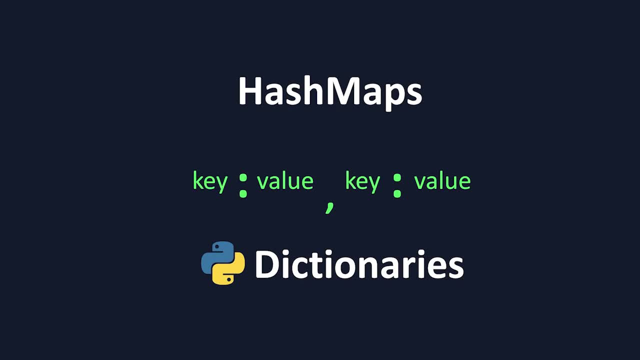 them up with unique identifiers called keys. A simple example to understand this is a university GPA directory. A simple example to understand: this is a university GPA directory called keys. A simple example to understand this is a university GPA directory called keys. Each student likely has. 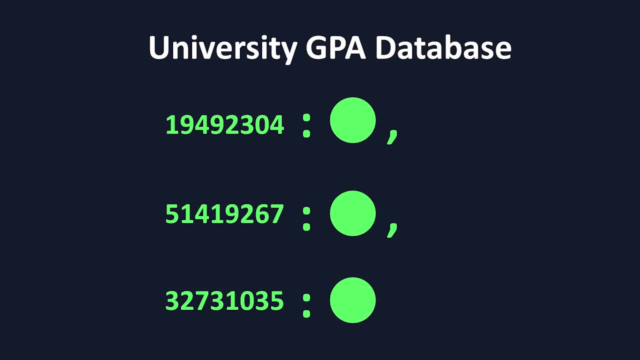 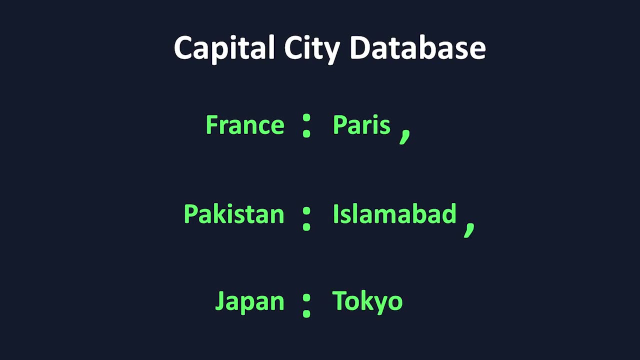 a unique student ID, which is the key, and it has a respective GPA along with it, which is a value. Or think of a list of capital cities. If we make the keys countries, we can just look up the country to find the capital city, which is the value. Hash maps are useful for two main reasons. 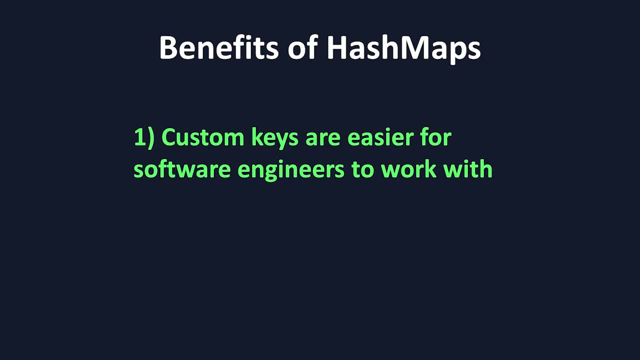 The first is when, working with big software systems, readability becomes incredibly important and being able to read the data is a key. The second is when, working with big software systems, being able to read the data is a key and being able to customize keys can be quite helpful. 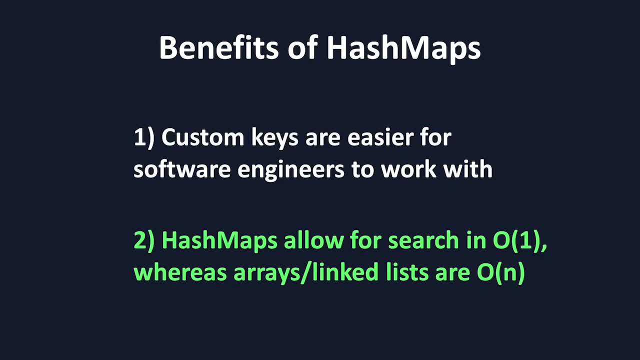 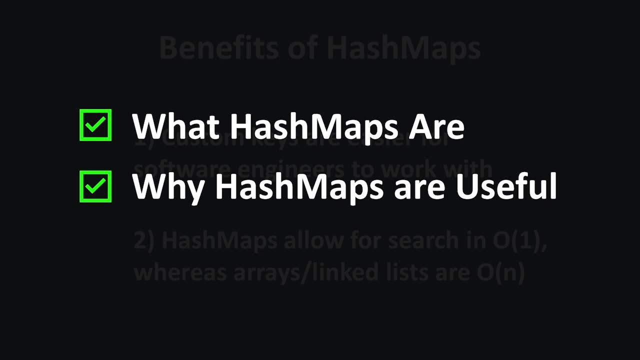 The second is that hash maps allow for searching of specific values in O run time, Which is faster than Arrays and linked list, which have a search time complexity of O. Now you know What hash maps are and why they're still useful, But let's dig deeper and understand how hash maps 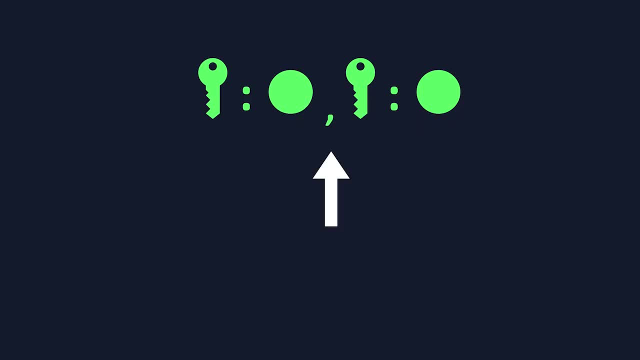 actually work. Hash maps are commonly built off of a predefined data structure like an array. To survive without hash maps, you have to navigate a database called an array. Like hash maps, hours are more valuable than hours. With hash maps, a specific number of units takes on a 25% operation, whereas subn Republican also. 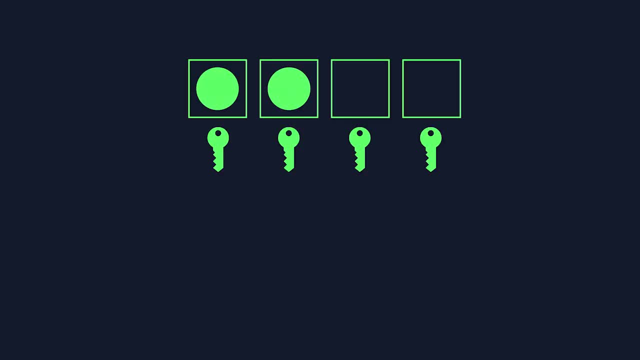 arrays do also have keys that store values For arrays, though the key is a preset number called an index, which starts at zero. A hash map is created from an array through the use of a hash function, which takes in a custom piece of data that we want to assign to a key, like a country from our earlier example. 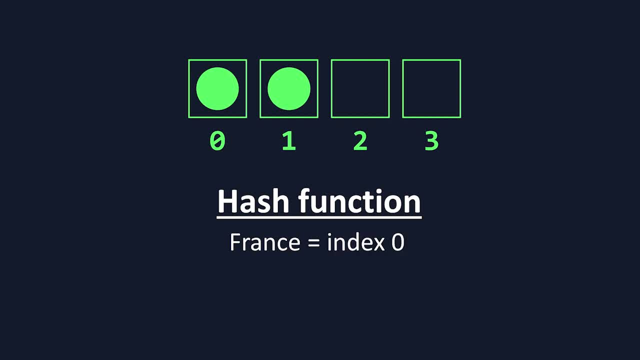 and maps this data to an index on the array. These hash functions can get complex, especially as they have to tackle issues that come up when mapping data to indices. The most common issue that comes up is called a collision and occurs when a hash function tries to assign a piece of data to an already 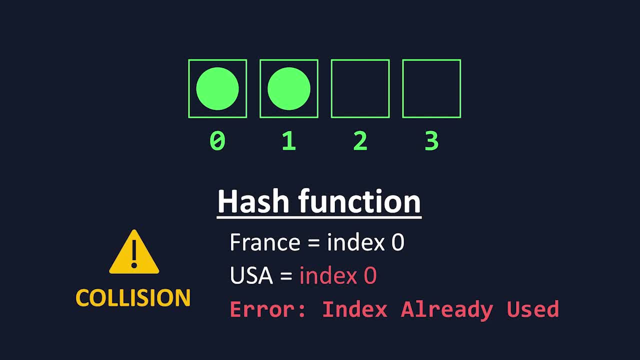 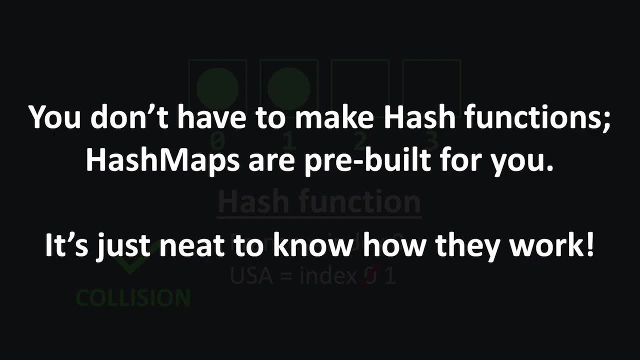 used index. In this case the hash function, has to have some efficient way to reassign this data to a different, non-used index. Hash functions are a bit outside of the scope of this video and in almost all modern programming languages hash maps are already implemented. 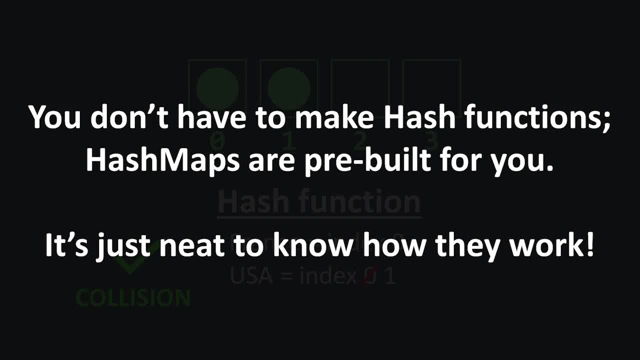 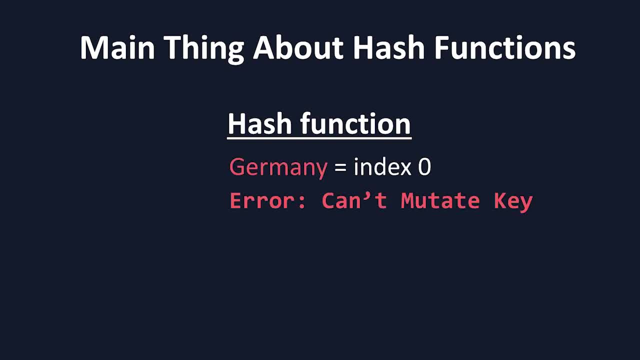 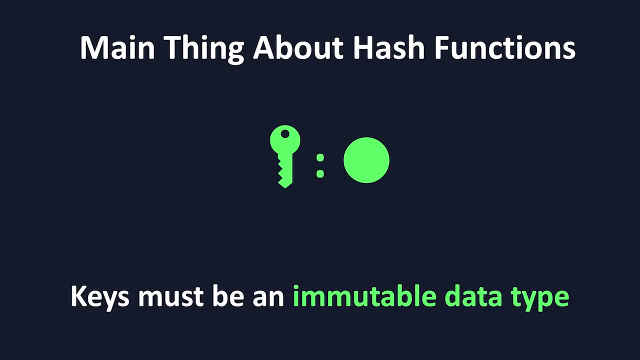 So you don't have to worry about building them yourselves. The one thing you should know about hash functions, however, is that once they map data to a key, they cannot change this key. This means that any key in a hash map must always be immutable. If you try to assign a mutable type of data as a key, such as 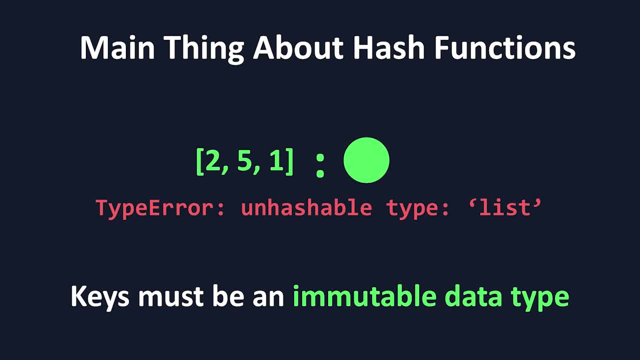 an array, you will get a type error that says unhashable type. If you see this error, it means you tried to assign a mutable data type to a key. To fix this, simply convert the data type to something that is immutable, As we got. 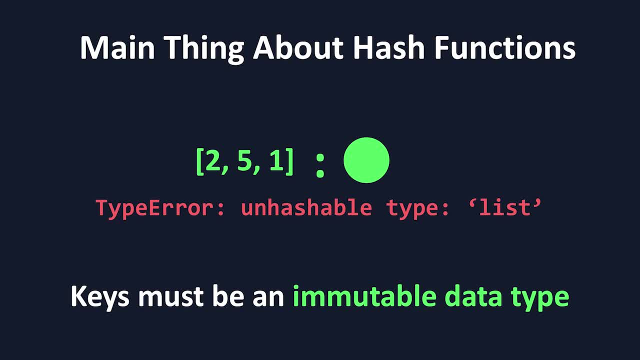 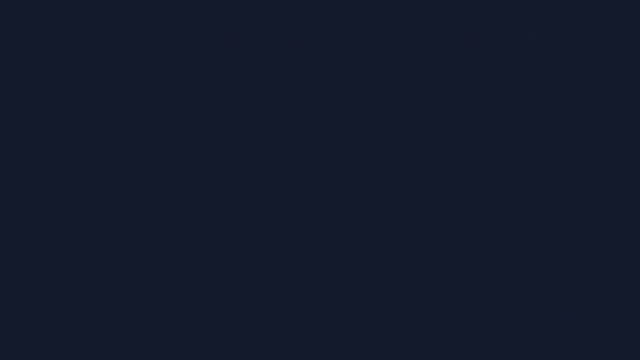 the error from using an array. our solution would be to convert it to a tuple, which makes it immutable. Now this tuple can be used as a key. Hopefully it's all coming together and you can start to understand why hash maps are efficient. If we used an array for our capital city to country scenario, we 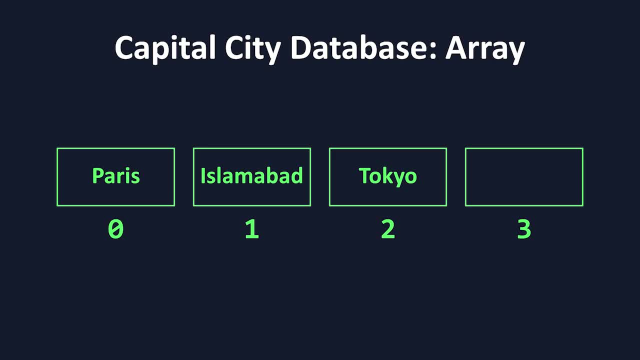 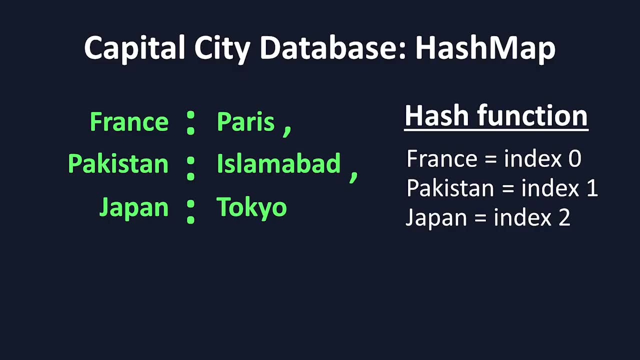 would have to make something like this For a program to find a capital city. they would have to search through an array of different types of hash maps. To do this, you'd have to find a label that says to search through every single index until they reach the correct value With a HashMap. 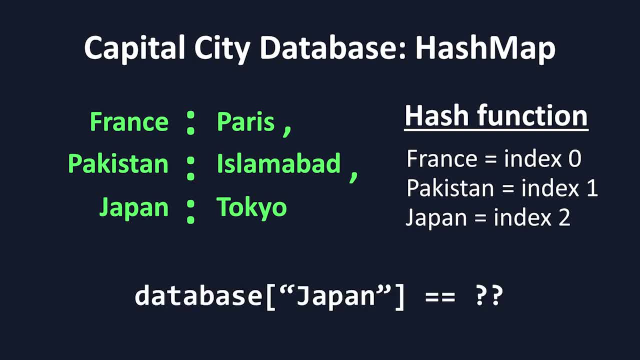 the program just has to receive the country name. From here, it can put the country name into the hash function, which spits out the right index without needing to go through every element in the list. It's time for us to look at how HashMaps are actually implemented In many languages. 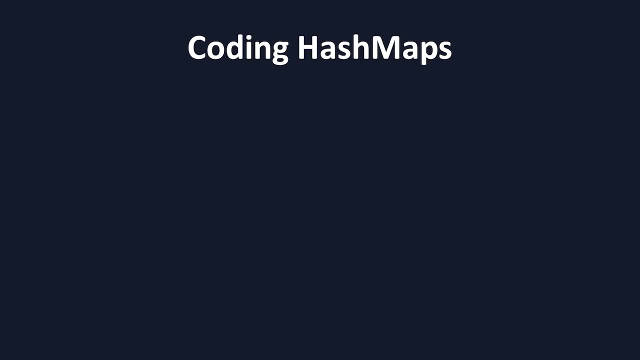 HashMaps have different names. When it comes to Python, HashMaps are called dictionaries, but I generally refer to them as HashMaps. anyways, We first create a HashMap by initializing it. Let's call ours CityMap. We can initialize it in either of these two ways. 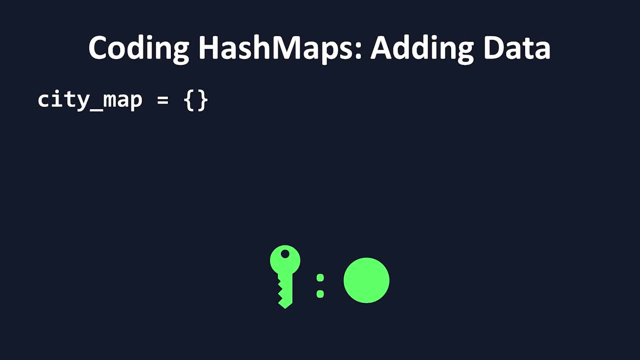 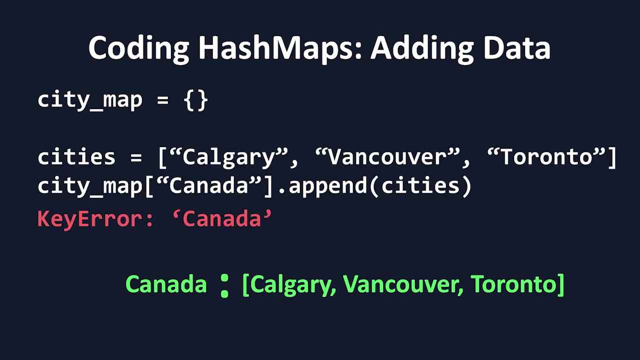 Now let's add our first key-value pair. I want to add in Canada as a key and have an array of cities as values To do that. this is our syntax. Oh no, we got a key error. Why did this happen? 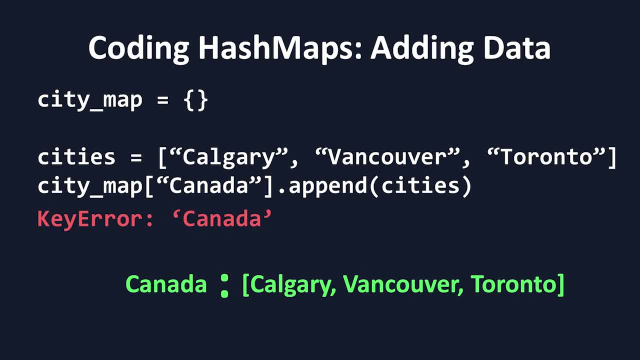 This is a very common mistake people make with HashMaps. We tried to assign the three cities to the key of Canada, but that key doesn't exist in our HashMap yet, So we first need to initialize this key. Now we can add these cities to this empty array. 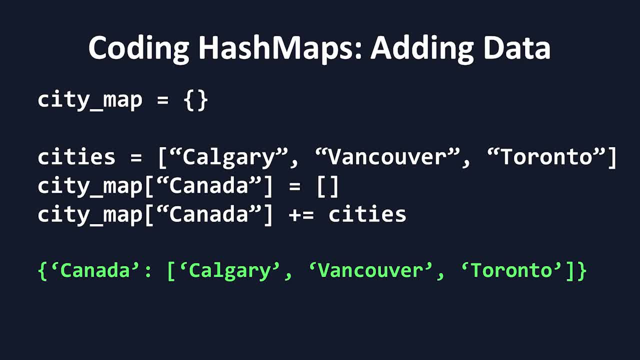 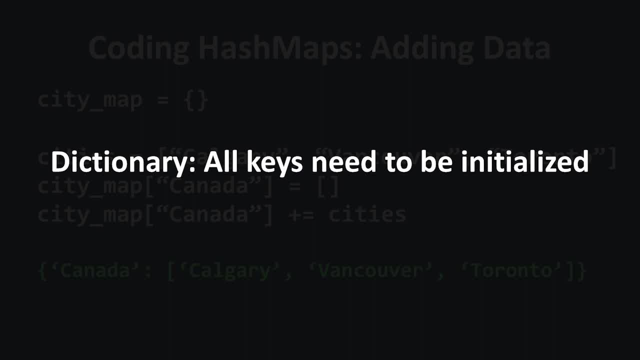 And this is what our result will look like after this. Here's a neat trick: To avoid having to initialize an empty array for your keys every single time, we can use a specific type of Python called a default dict, which will have an empty array or other type of data assigned to a. 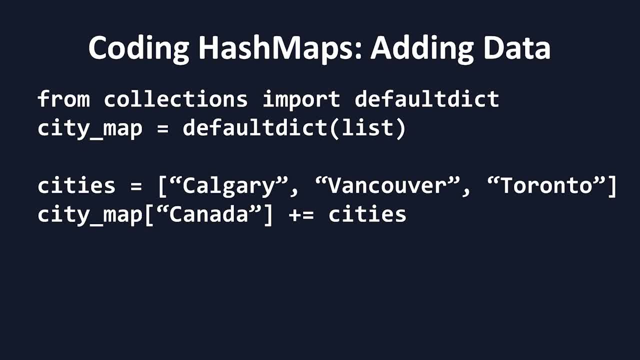 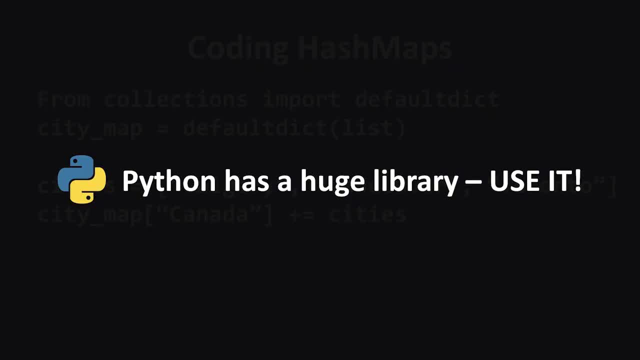 key by default. Here's what the code would look like if we chose to do it this way. One of the reasons Python is awesome is because of its huge library, and this is a prime example of this. I highly recommend taking advantage of default dicts for solving coding problems. 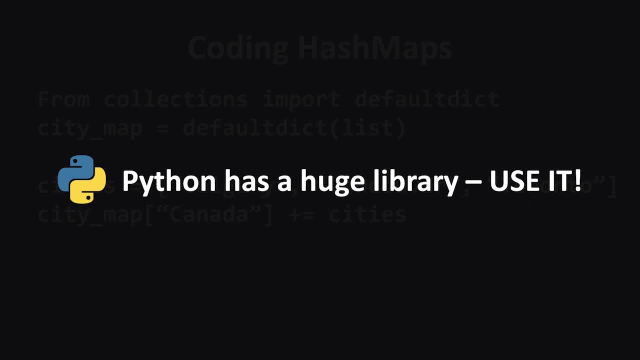 as it's an incredibly useful feature that will help you avoid unnecessary mistakes. The other major thing you should know about HashMaps is that it's a very easy way to initialize your code. If you're not familiar with HashMaps, you should know how to retrieve information from them. 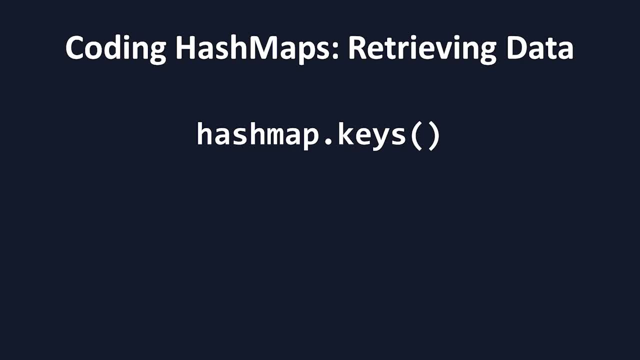 There are three methods for this: keys, values and items. The keys method returns all of the keys from the dictionary in the form of a list. values method works very similarly: returning all of the values of the dictionary in the form of a list. 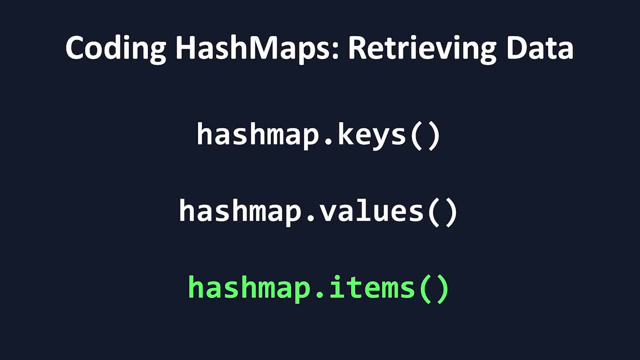 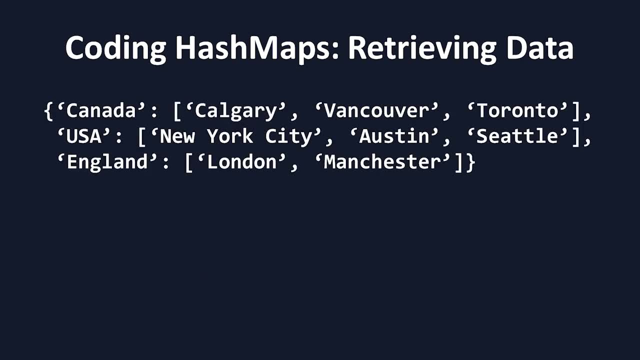 And items is a combination of the two. It returns a list of all of the key-value pairs as tuples. The keys method returns all of the keys from the dictionary in the form of a list. As you can see, it now has multiple countries and cities. If we wanted to get a list of only 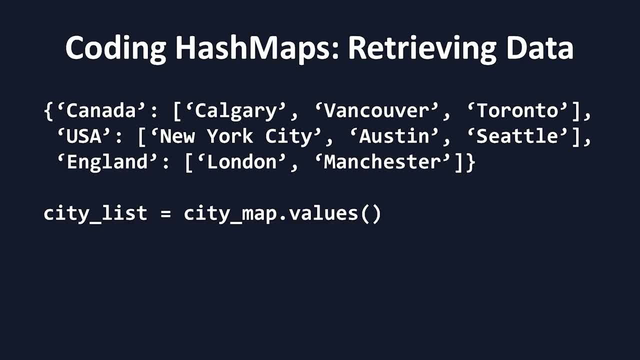 the cities. we could do so by calling the values method like this: Now we have a list of cities in city list that we have extracted from the HashMap. Great, now that we've learned how HashMaps work and how to code with them, let's use our new knowledge to solve a popular coding interview. 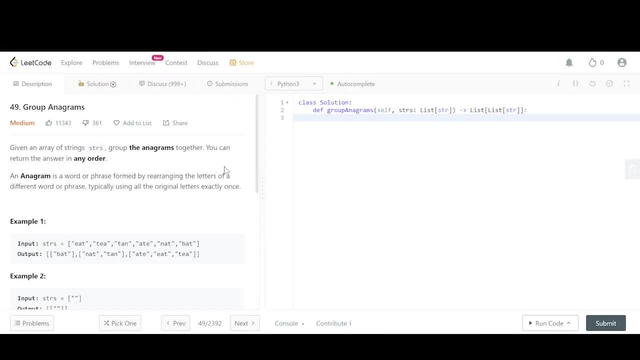 problem. The question we are going to be taking a look at is Leap Code 49.. We are given an array of strings and our goal is to return an array that groups all of the anagrams together. If you don't know what an anagram is, it does give a little explanation. 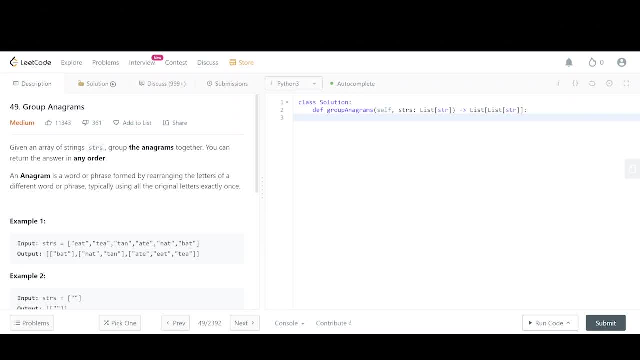 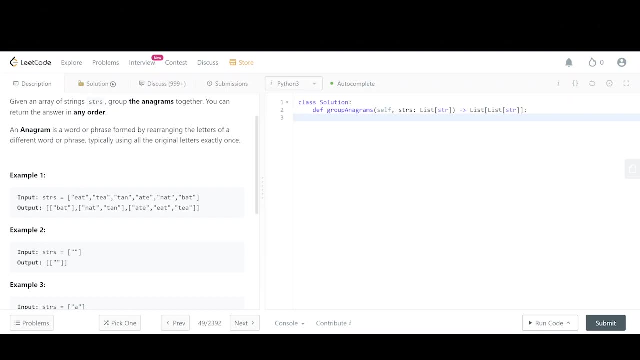 Basically, an anagram is a group or pairing of words where all of the words have the same amount of letters. Let's take a look at example 1 to understand this a bit better. As you can see, we are given 6 different words in the strings array. 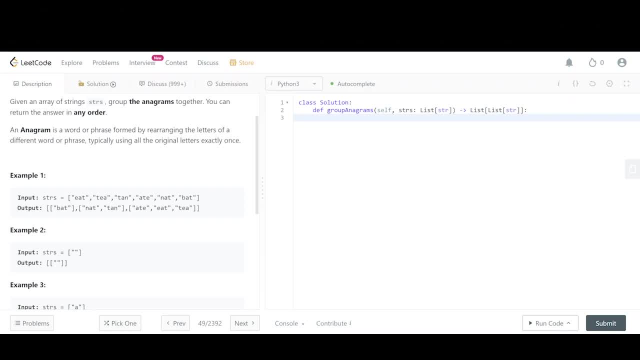 bat is put on its own because it is the only word in the group of 6 that has 1a, 1b and 1t. nat and tan are grouped together because they both have 1a, 1n and 1t. 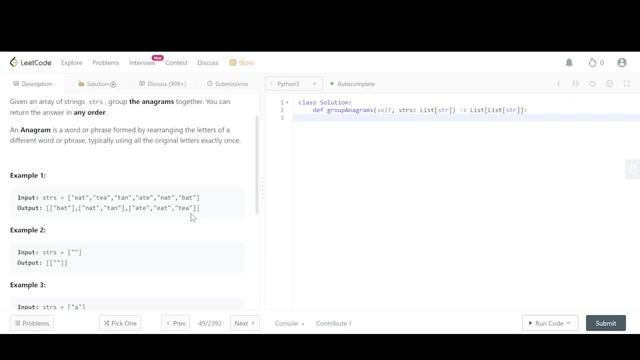 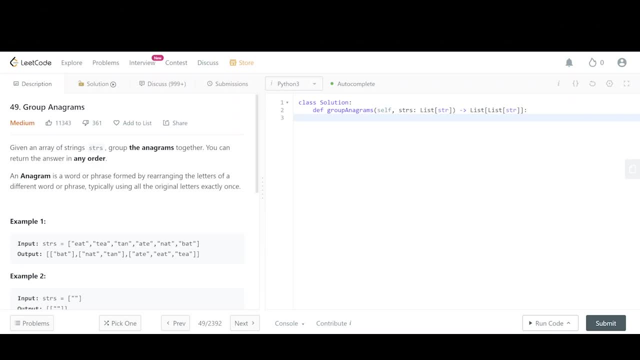 and the same thing goes for 8,, eat and t. Okay, great, now we understand the problem. How do we solve this? Your first instinct might be to think that we should go through each of the words in strings and compare that word with all the other words. 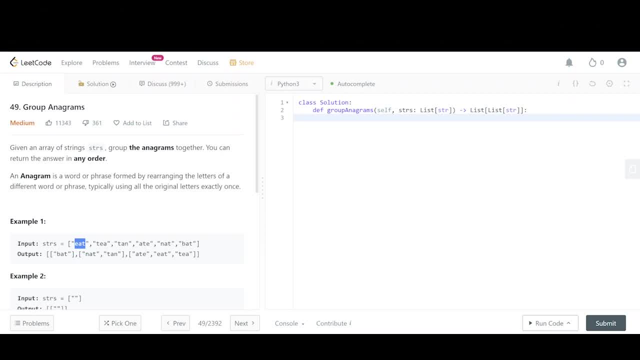 So, for example, we can start at eat and check: okay, it has an, a, an e and a t. What about t? Oh, they have the same letters. let's group them together. Now let's compare eat and tan. 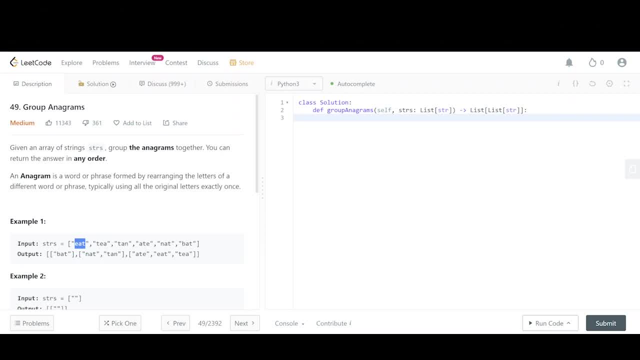 and go through them that way. However, if you did that, it would become incredibly inefficient as the the length of strings got longer, because we have to check for each element in strings. we are checking every other element. This has a time. complexity of n. 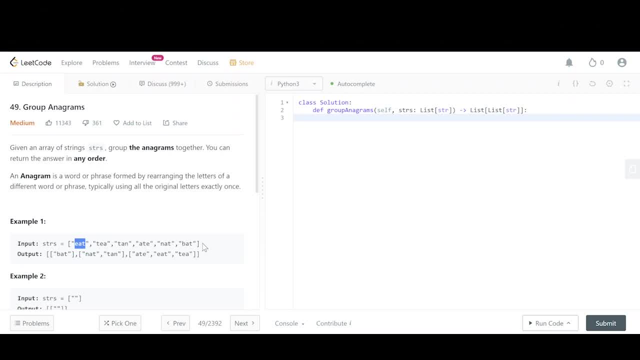 squared. What if there's a more efficient way of doing this? I'll give you a few seconds to stop and think about how we can go through this a bit better. Now we've come up with an idea for how to solve this in O of n? squared time, but 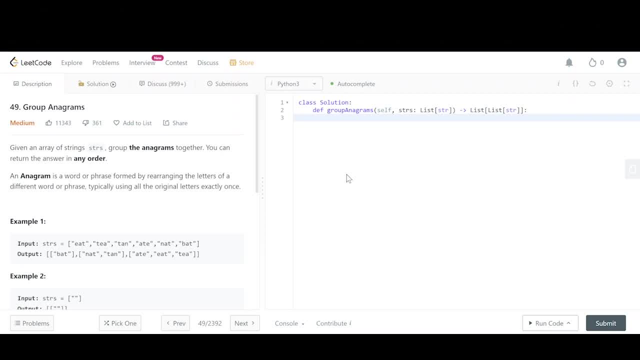 can we make this better? What if we could go through each element only once and check if it's an anagram from there? That would be a solution in O of n time. Seeing as this is a video on hash maps, you've probably already started thinking. 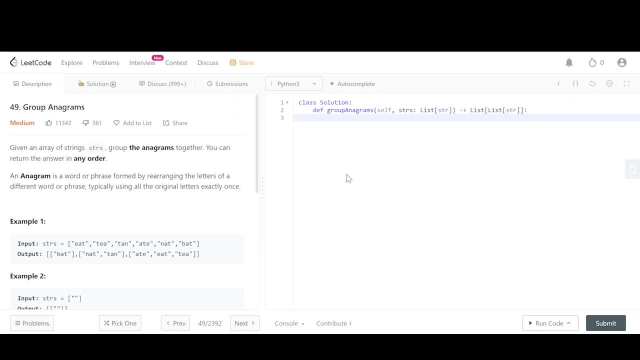 that we could use a hash map to solve this. If you're on that train of thought, you're absolutely correct. but how are we actually going to be using this hash map? I'll give you a few seconds to think about that. Okay, if you need more time, and pause it here, but now we're going to go through. 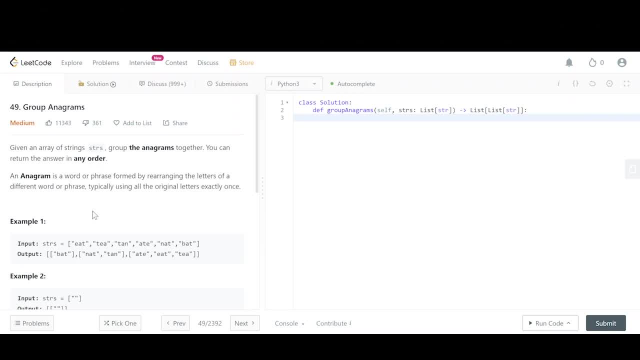 the solution. Basically we want to go through each word in the strings and check if its combination of letters is already a key in the hash map. So we would get to eat and check: is the combination of 1a, 1e and 1t a key in? 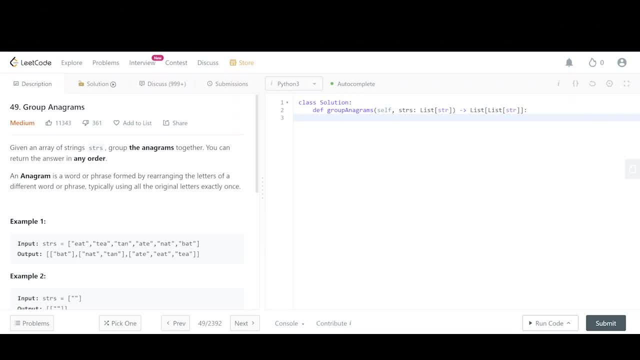 the hash map. If it is, add this word eat to the array associated with it. with that key, Then let's check t. Is e, a and t already in there? Yes, it is, we just saw it. So now let's add a t as another value in that array associated. 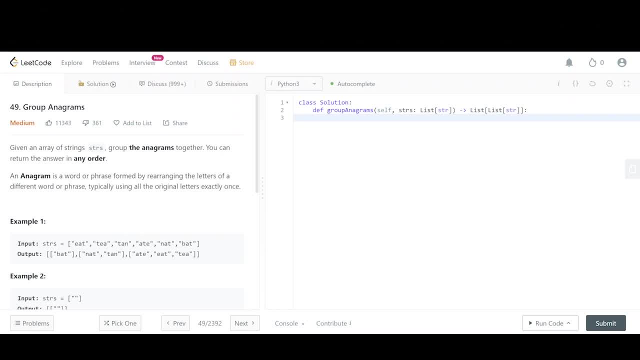 with that key. This process will continue until we've built out a full hash map. From here, all we have to do is go through each of the values in the hash map and append them to our array. So let's get started on the coding process. 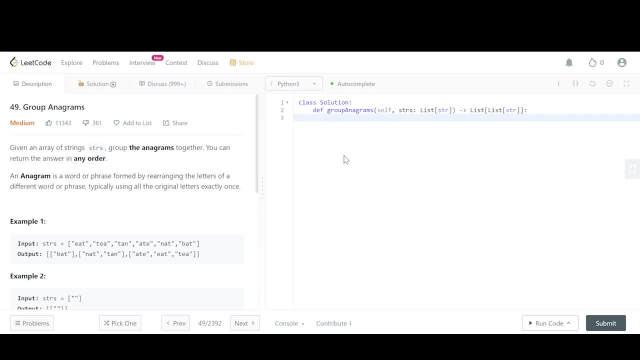 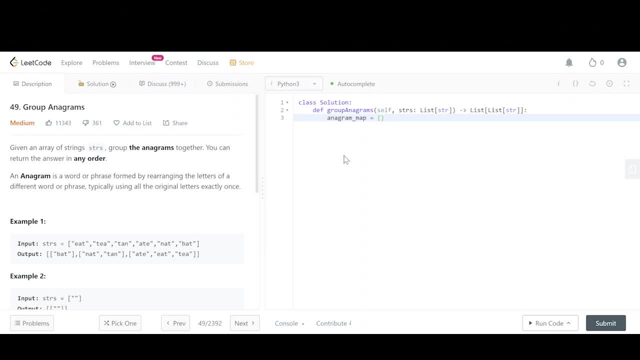 of understanding what it does. We also know that our result has to be an array, So we're going to be creating a result as an empty array for now. We'll be adding values to it later. The first thing we need to do is go through each. 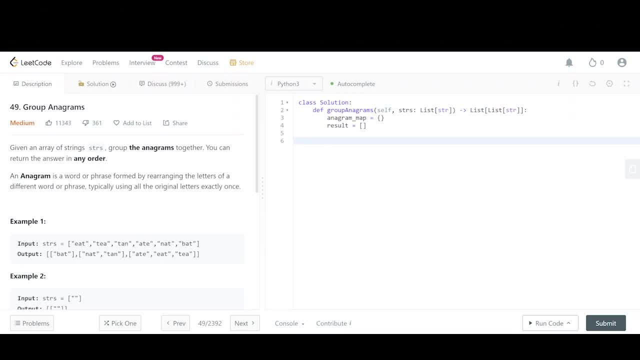 of the words and check if it's an anagram and for which anagram it is. we need to add that to the anagram map. So we'll say for s in strings, So for each string. Now how do we actually check if a word matches a key in the anagram? 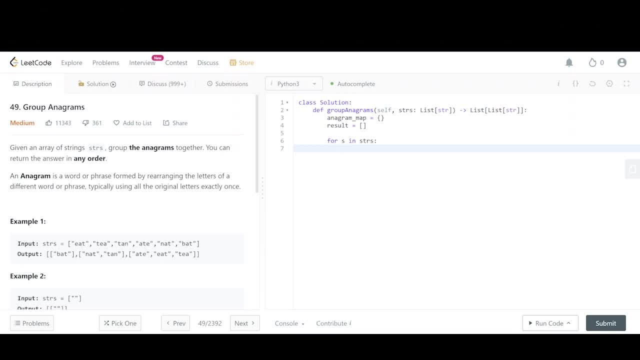 map, We could always go through each word and count all of the letters. but there's actually a simpler way. In Python you might be familiar using the sort method which allows you to sort a list of numbers either in ascending or descending order. But you can actually use the sort method on words as well. If we use the sort. 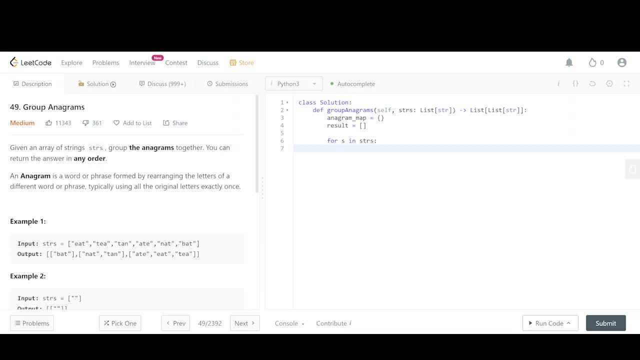 method on a string. it will sort that string in alphabetically increasing order. As you might be starting to find out now, this is how we're going to solve this For each of these words, if we sort them in alphabetical order. all of the 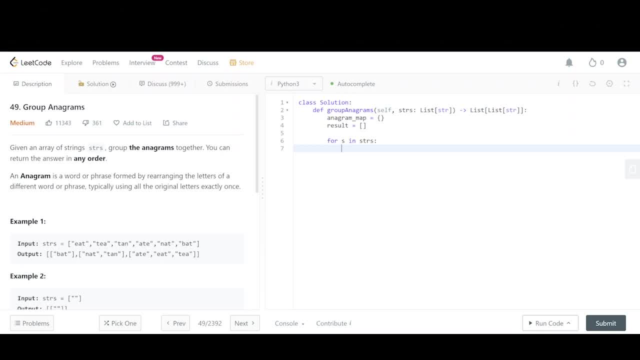 anagrams will end up being the same combination of letters, So in this case, with 8,, 8 and T, they will all be re-sorted as A-E-T. This will be our key in the anagram map. Now, once we have figured out what the sorted version of each of these words is, 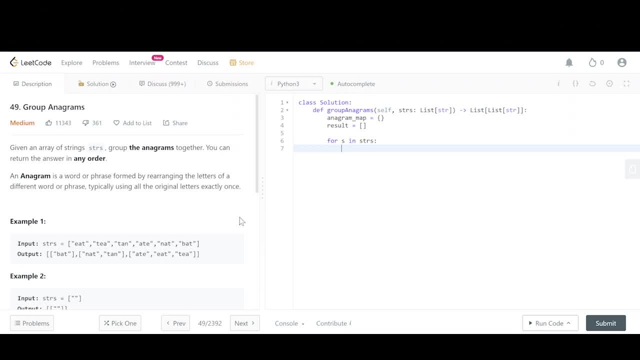 we know what the key is. All we have to do is add the original unsorted word to that key. So we are first going to sort the string and we will call ours sortedS, which is going to be a sorted version of that. 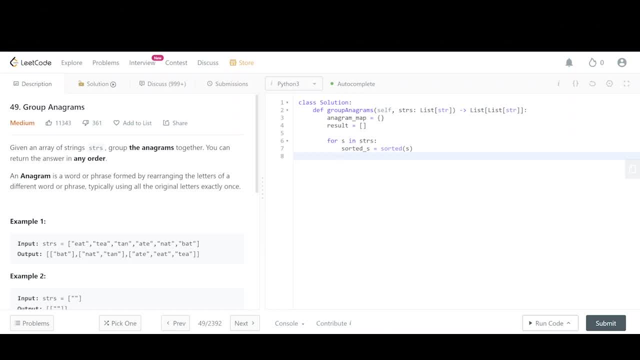 And then we are going to be adding that as a key into our anagram map. So anagram map and our sortedS is going to be our key. For this key. we want to append the original word onto the array. 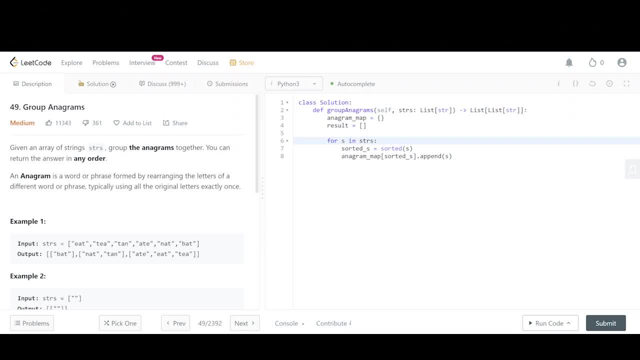 Now there are two mistakes here and I hope you'll understand why, And I hope you caught on to both, because they are the two mistakes we talked about earlier in this video. The first thing is we don't have this key initialized in our anagram map. 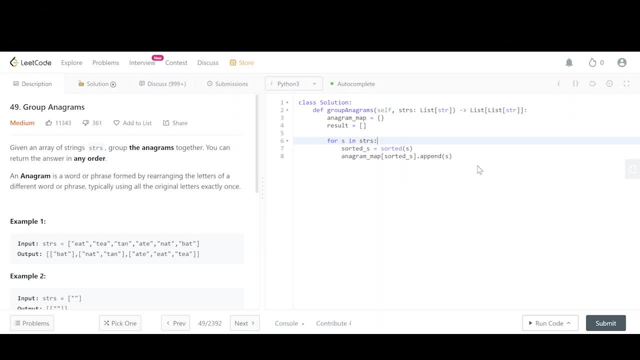 So we are going to get a key error. If you remember the way around this, we are actually going to be using a default dict. So we're going to come up here and we're going to say: from collections, import- default dict. 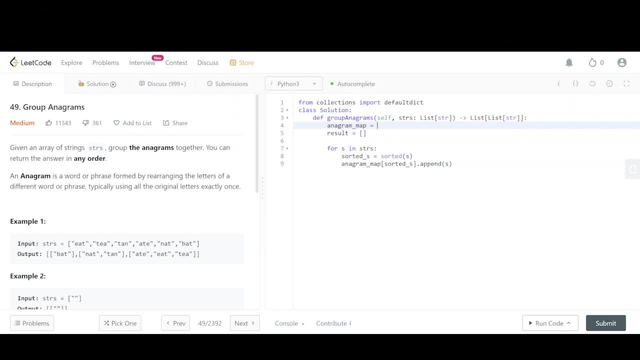 We're now going to be replacing the Python standard dictionary here with a default dictionary, And the type we want to set it to is list. This just means that for each key that we are going to be adding to our anagram map, we want the default value to be an empty list. 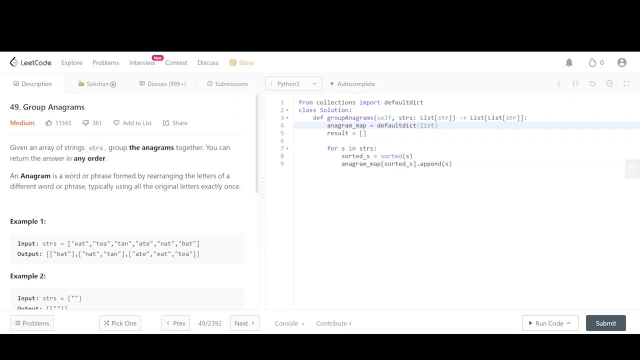 You could do the same thing with integers, strings, etc. It's just in this case we're going to be using lists because we're appending things to them. Great, that's mistake one Mistake number two is that we are using sortedS. 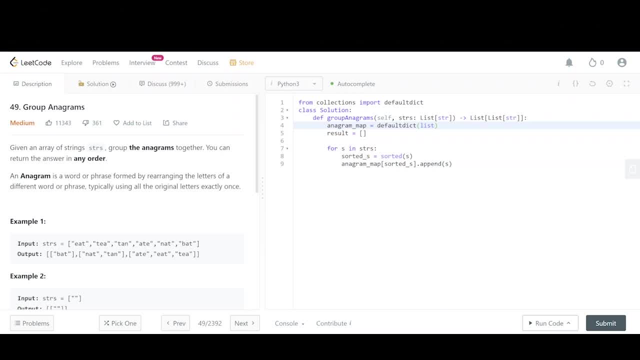 as our key. However, when you run the sorted method on a string, you're actually getting a list object back And, as we talked about earlier, lists are mutable And mutable data types cannot be keys. So to get around this, what do we do? 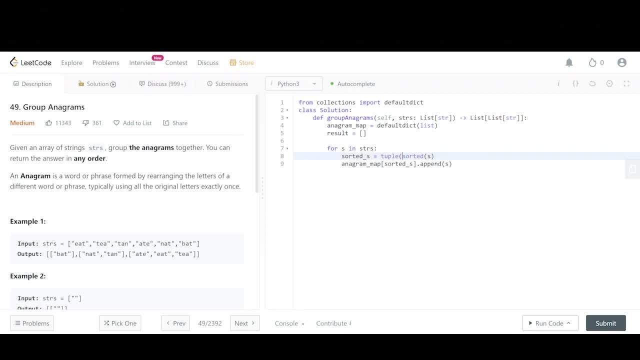 We simply need to convert this list into a tuple, which is an immutable data type. After we have done this, our anagram map will come together. Just to see what that looks like, let's print out our anagram map. As you can see, it is a default dict. 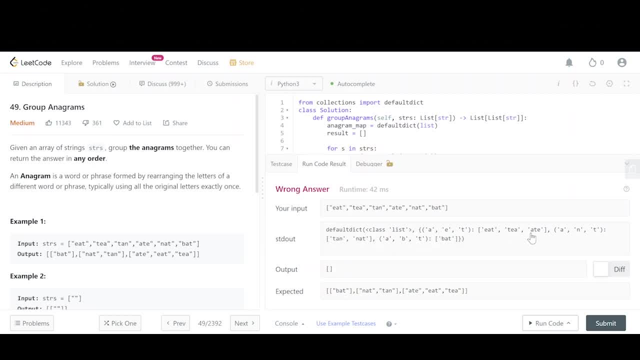 where a, e and t has these three words: a, n and t has these two, and a, b and t has bat. Great, now that we've done that, we're really close to the solution. All we need to do now is just add: 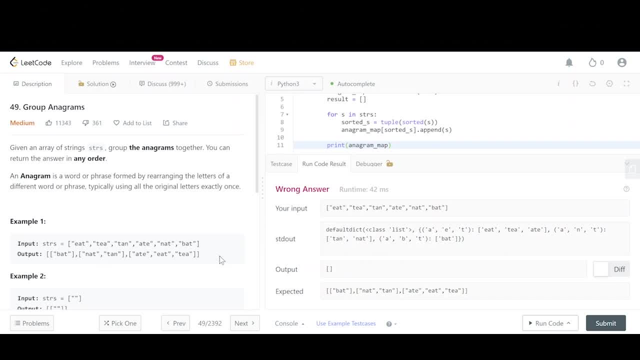 all of these values and append them onto the result. To do that, we want to go through each value in the HashMap. So we're going to say forValue in anagramMapvalues, which anagramMapvalues will give us a list of the values. 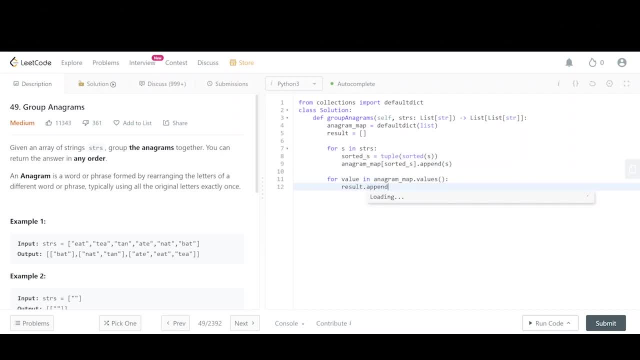 And for each of these values, we are just going to append them to the result. After we've done that, all we have to do is return our result and when we call the function, exactly Just like that, we solved it Now, as you can see the output and expected answers. 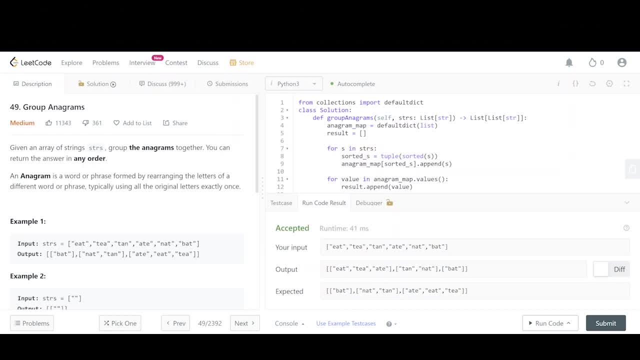 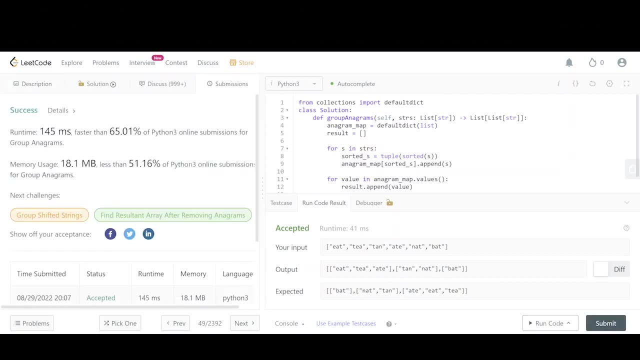 are actually a little bit different, but that is because the question says you can return the answer in any order. If we submit this, you should see a success message. There you go. You've officially used a HashMap to solve a medium level leak code question. 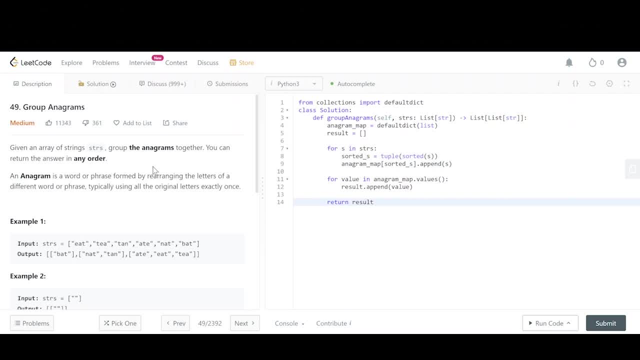 Now I know it may have seemed a bit complicated at the start but, as you can see, if we walk through it kind of step by step, and you understand how HashMaps work, you can start to see where they're applicable and how they can be used. 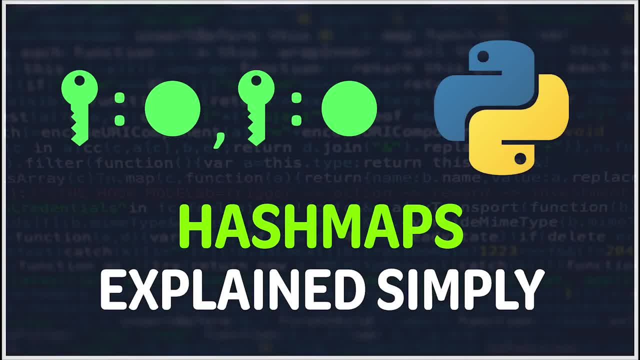 to make problems more efficient. Thanks so much for watching. I hope you enjoyed the first video in this series. I'll be working a lot on this series in the coming weeks, so you'll have everything you need to prepare for coding interviews. Please like subscribe. 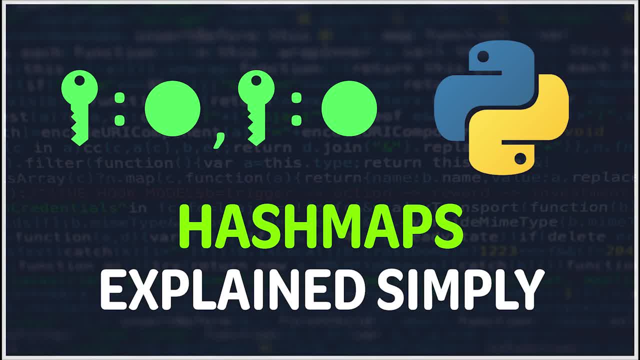 and comment if you enjoyed this video. Each like, comment and subscription makes a huge difference, so I'd really appreciate if you can do that, as well as share it with some friends. Thanks and see you in the next one.